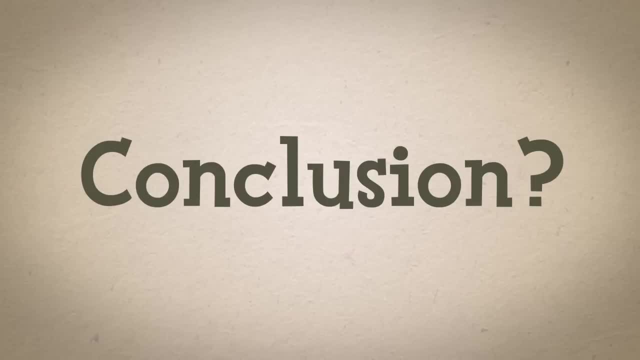 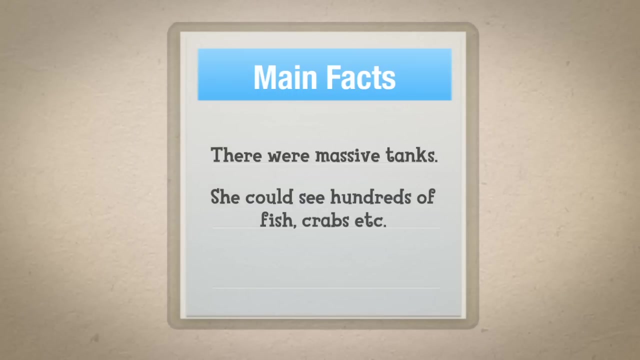 Where is Shruti? What conclusion can you draw? Was she swimming in the ocean? Was she visiting an aquarium? First ask yourself what are the main facts. There were massive tanks. She could see hot water. There were hundreds of fish, crabs and other amazing ocean creatures around her. 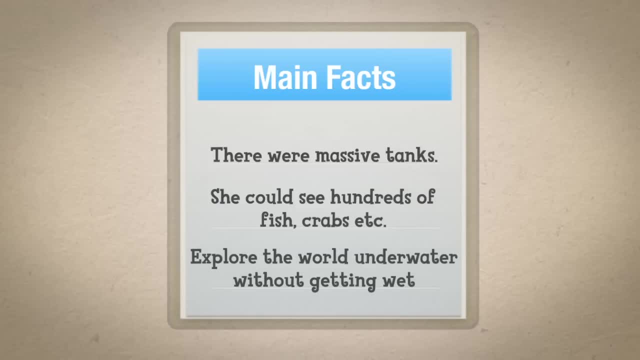 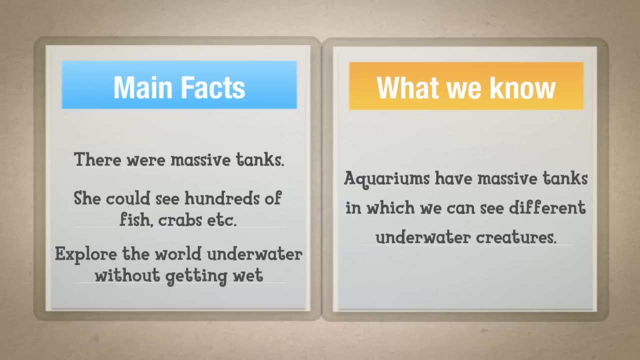 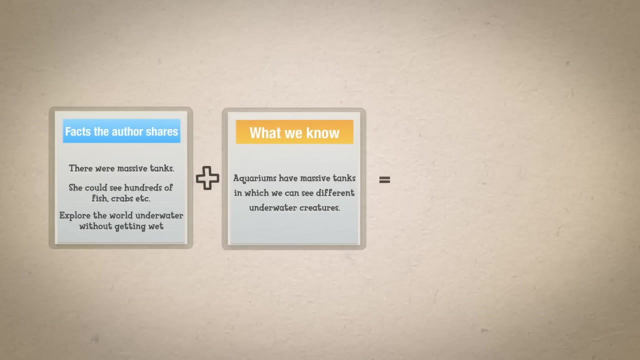 She could explore the world's underwater without getting wet. What we know. Aquariums have massive tanks in which we can see different underwater creatures. So first we must take facts that the author shares plus what we already know, equals drawing a conclusion. 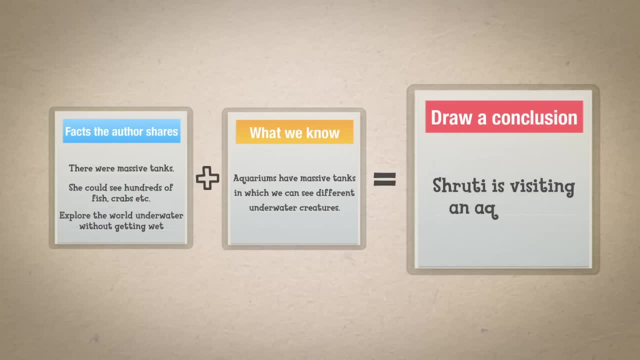 The conclusion we can draw is that Shruti is visiting an aquarium. When you read, you look for clues to help you decide what is happening in the story. Sometimes the author doesn't tell you everything that is happening. You have to think about the facts given plus what you know to draw a conclusion. 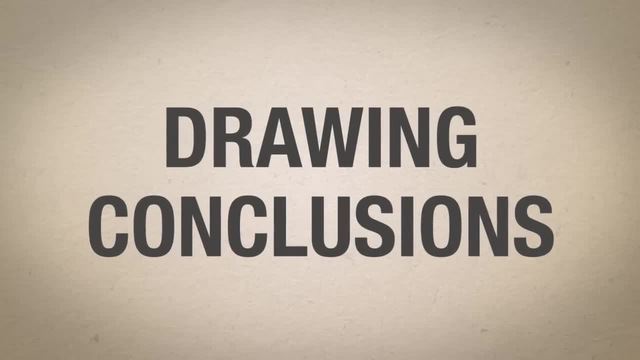 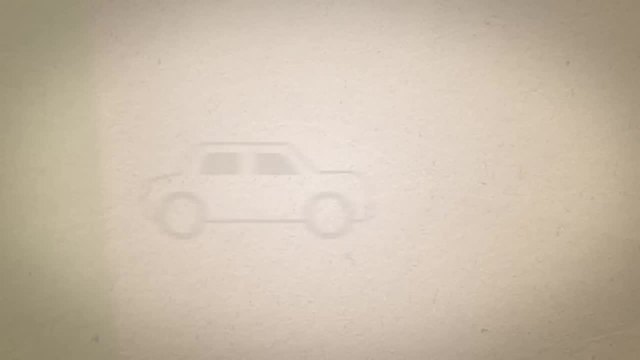 Drawing conclusions helps us deepen our understanding of what is happening in the story. Let's look at another example. Ram heard his mother blow the car horn. He ran down the stairs, Slipping on his t-shirt as he ran. What conclusion can you draw from what you just heard? 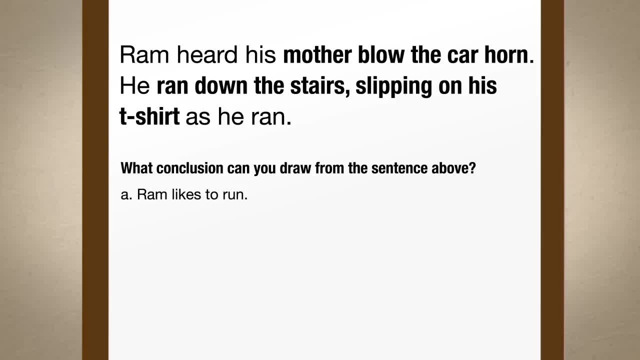 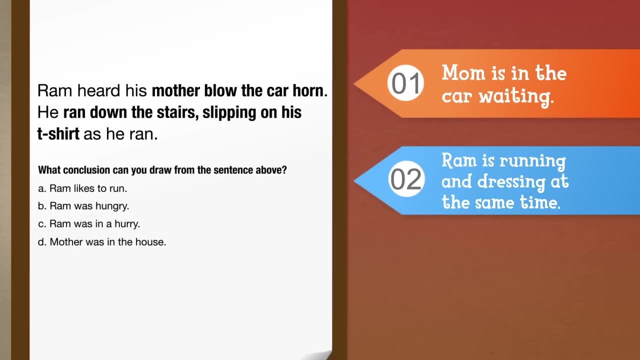 A Ram likes to run, B Ram was hungry, C Ram was in a hurry Or D Mother was in the house. When we piece together the facts: 1. Mom is in the car waiting. 2. Ram is running and dressing at the same time. 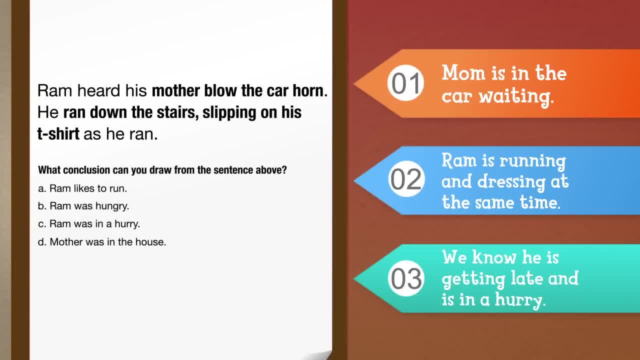 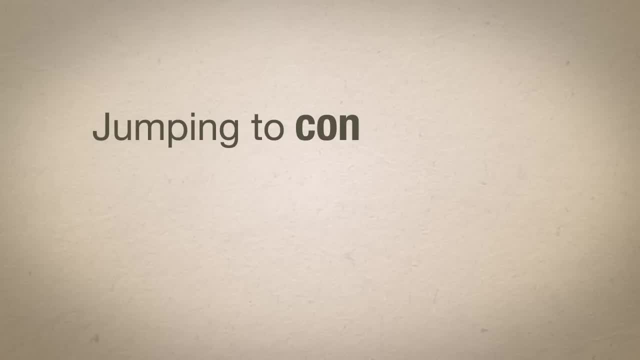 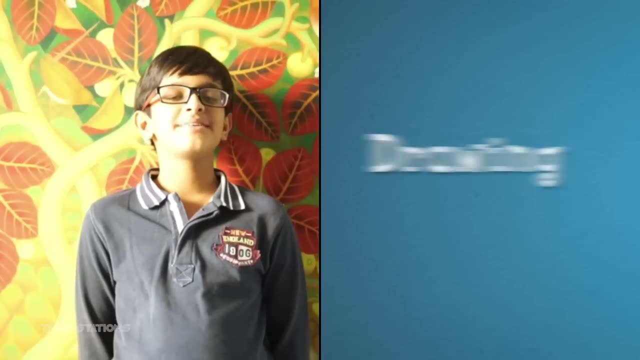 Then we know he is getting late and is in a hurry. But be careful, Don't jump to conclusions. Jumping to conclusions is basically making a conclusion without knowing the full facts. Thanks, Muzali. Drawing conclusions is basically using facts from the text with what you already know to 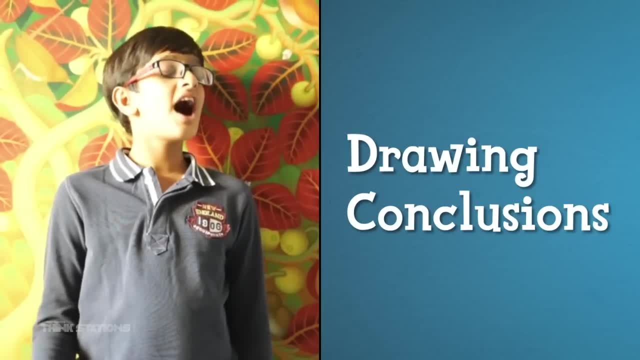 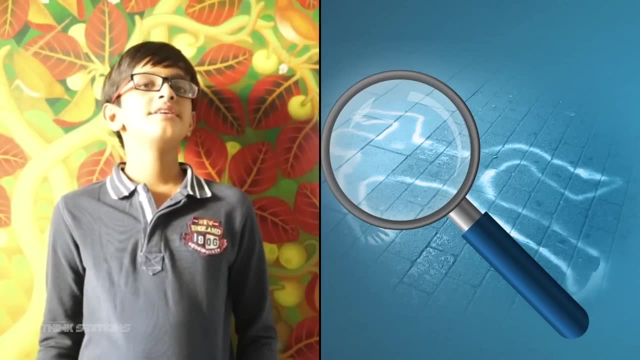 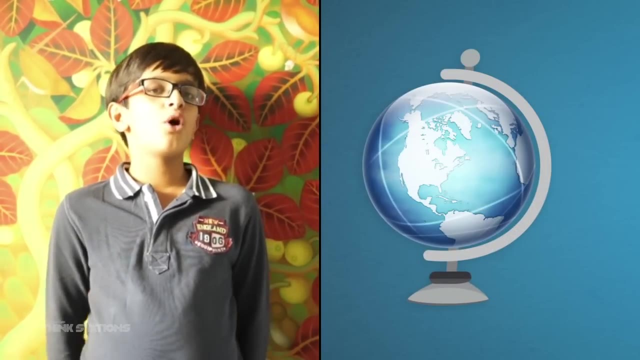 make a final decision. It's kind of like solving a mystery. You put together all the facts with what you already know to make a final decision. The more you know about the world around you, the better you get at drawing conclusions. Let's try an example.